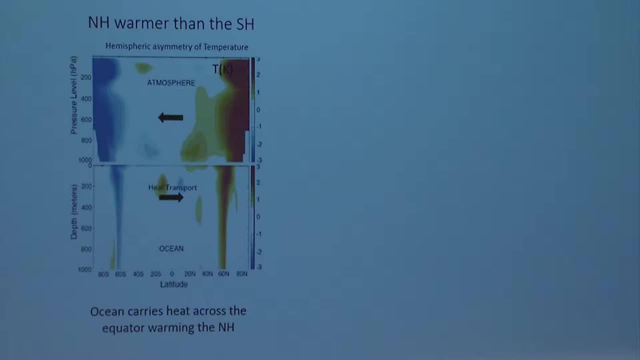 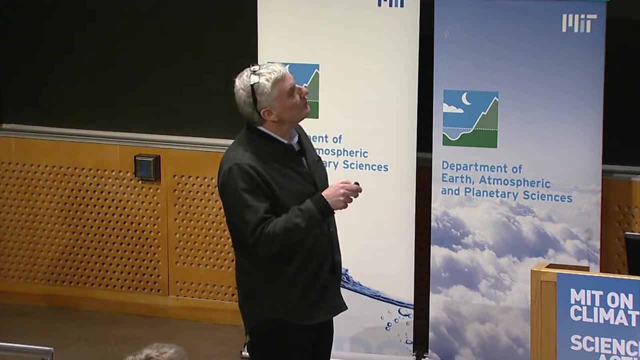 This is at the surface, This is the atmosphere and this is the ocean. So you can see that the northern hemisphere troposphere is 2 or 3 degrees warmer than the southern hemisphere troposphere And the northern hemisphere ocean is warmer- slightly warmer- than the southern hemisphere ocean. 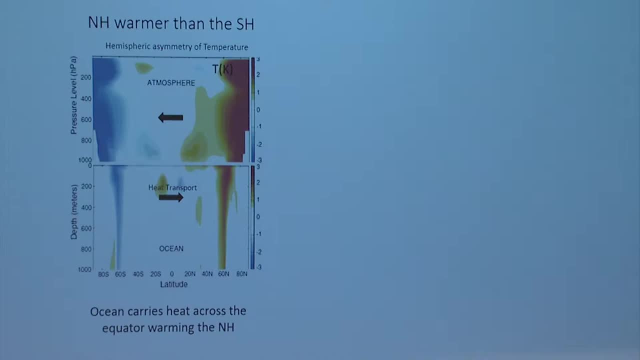 And what we think is happening? what we know is happening is that the ocean is actually carrying heat from the southern hemisphere and moving it into the northern hemisphere So that warms up the northern hemisphere troposphere. So the ocean carries heat across the equator, warming the northern hemisphere. 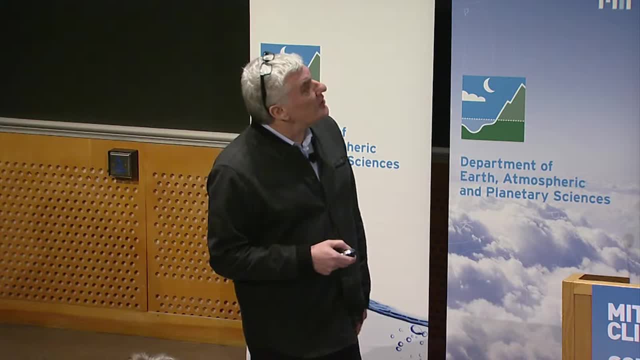 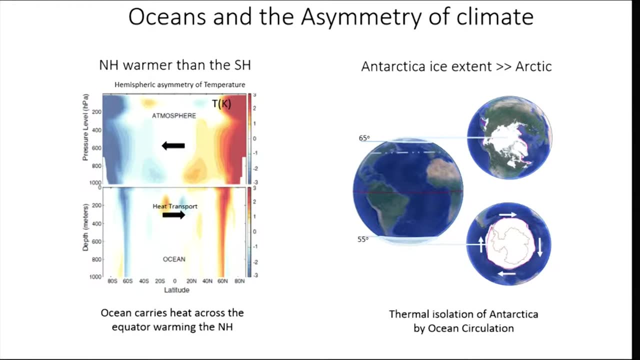 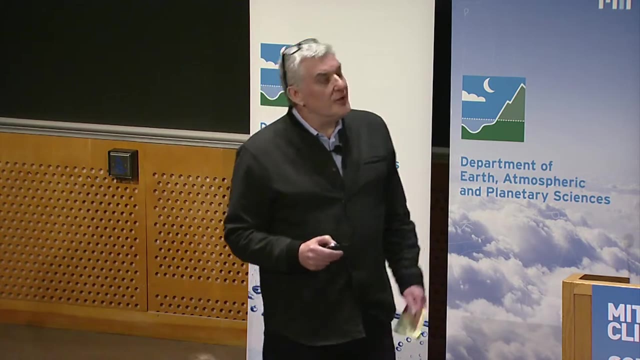 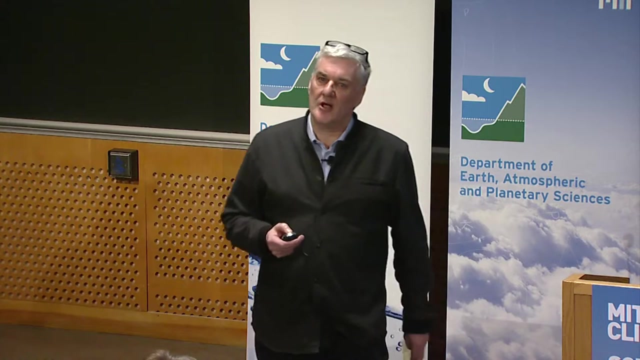 Another big asymmetry of climate is that there's a much more ice over Antarctica than there is over the Arctic. So there's 2 miles of ice around Antarctica, whereas the Arctic ice is much less extensive and we think might be quite vulnerable as climate changes. 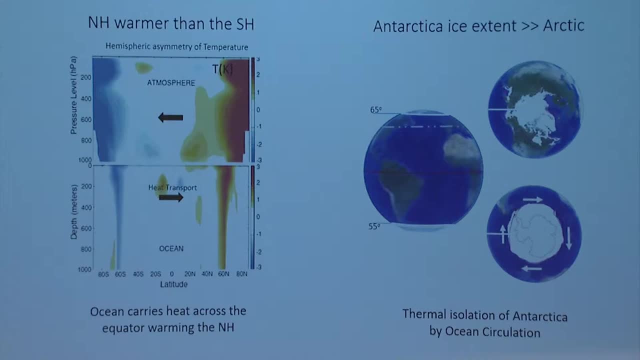 I don't think we should worry about Antarctica losing all its ice. It's not going to happen anytime soon. Big chunks of ice might break off and drop into the ocean, but it's going to be there. Now. one of the One of the roles that the ocean plays is that it thermally isolates Antarctica. 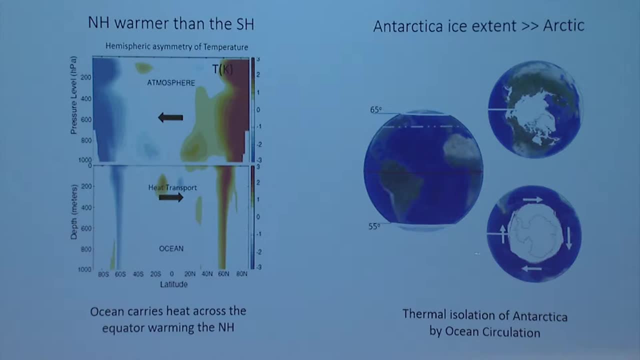 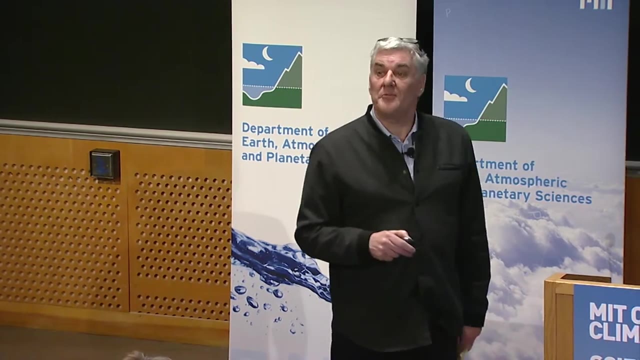 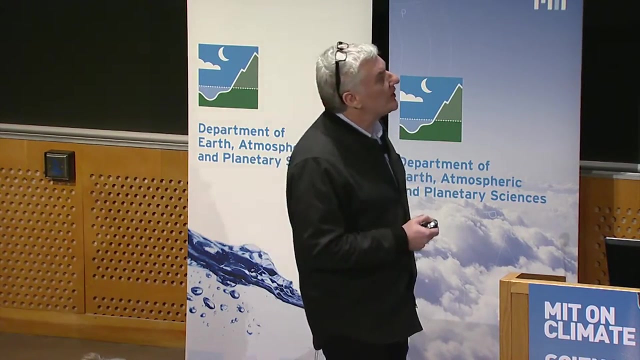 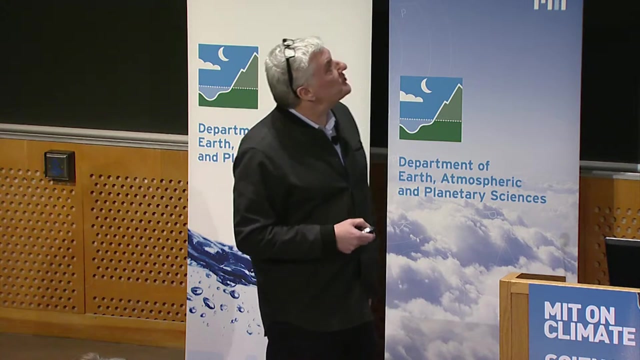 from the rest of the climate system because there's a circumpolar current moving around the southern hemisphere through Drake Passage And that thermally isolates Antarctica, enabling ice to build up. That's another important role that the ocean plays. Third, Another important aspect is the intertropical convergence zone. 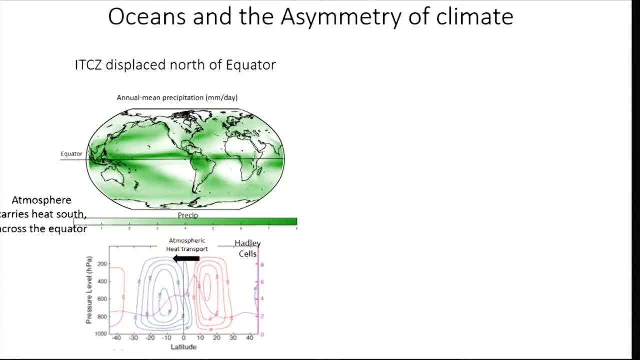 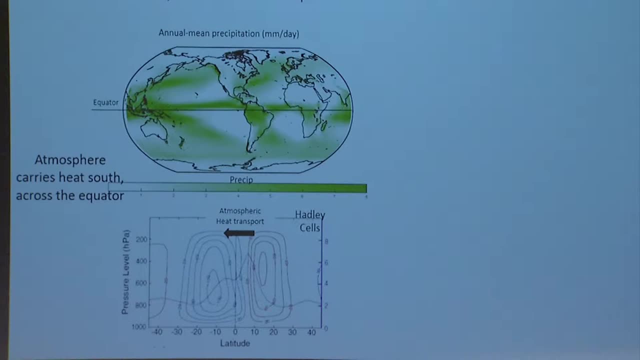 This band of precipitation is slightly north of the equator. This horizontal line is the equator and this is the annual mean precipitation in millimeters per day. It's slightly north of the equator, So the axis of symmetry of climate is not at the equator. 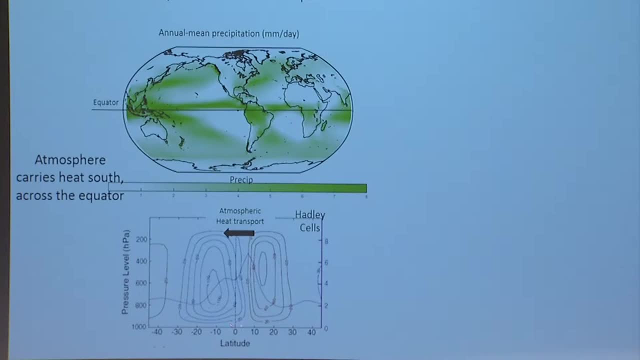 It's slightly north And if we go into the atmosphere here, this is the equator moving up into the atmosphere. These are the Hadley cells and there's rising air in this convergence zone which leads to all the precipitation And the Hadley cell is. 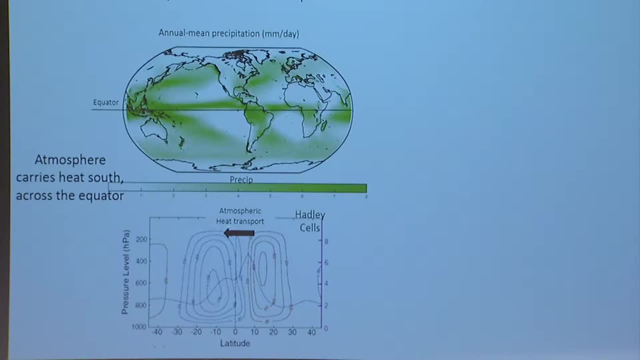 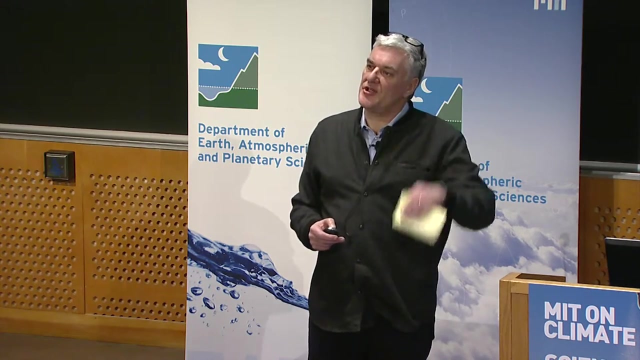 The rising is north of the equator and it moves southwards, And this cell actually carries energy from the northern hemisphere into the southern hemisphere. So the atmosphere is trying to equilibrate its hemispheric temperatures and it does that by shifting the axis from the equator north. 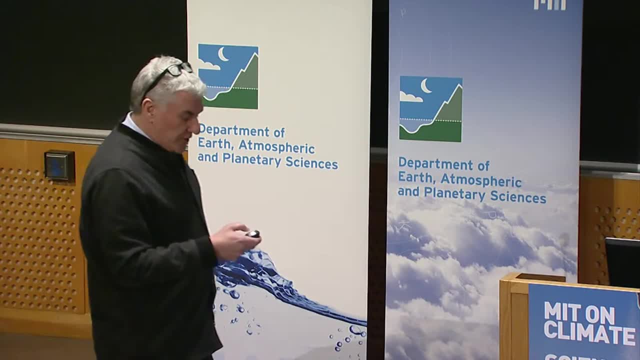 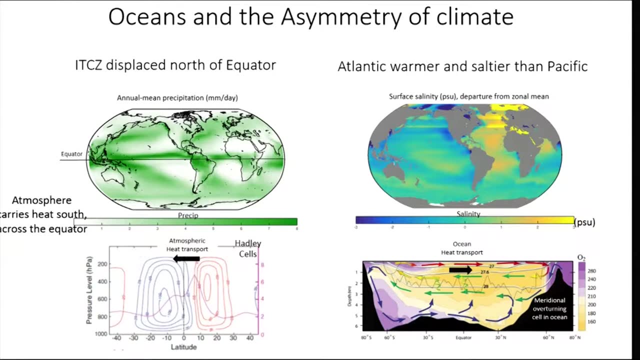 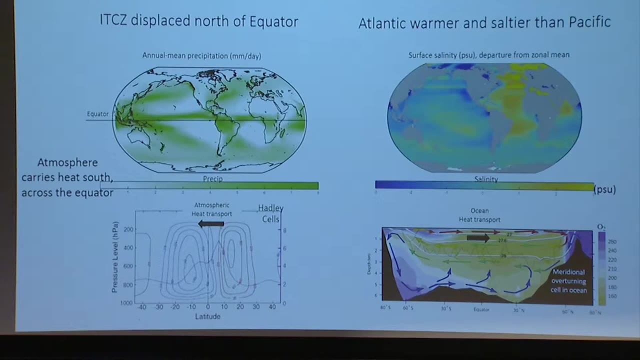 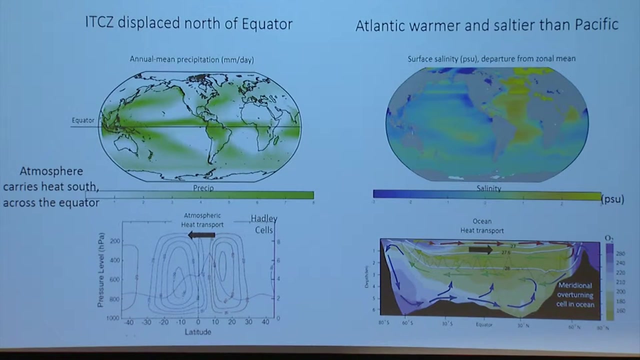 Another important asymmetry is that the Atlantic sector is warmer and saltier than the Pacific. So here this is the surface salinity, a departure from the zonal mean, and the yellow area are places where Tell us that the Atlantic is saltier than the Pacific. 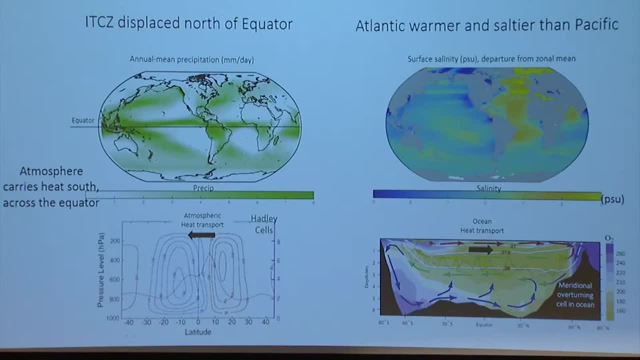 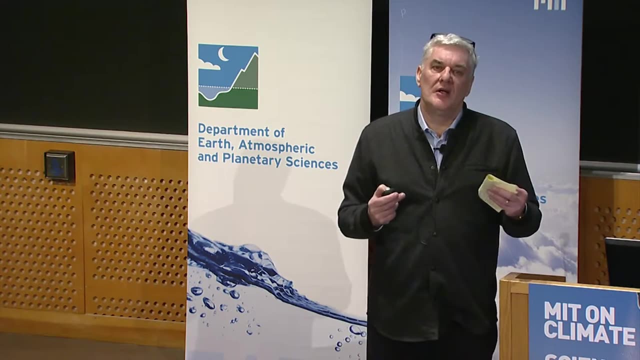 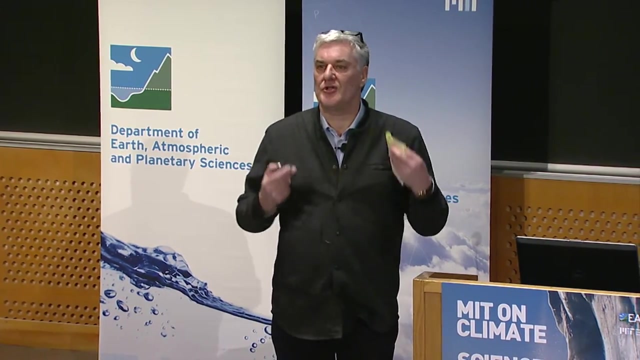 And this has a really important part of. This is a really important part of today's climate, because salty water is heavier, more dense than fresh water, And so you get in the ocean a big convective overturning cell, which we know as the ocean conveyor belt. 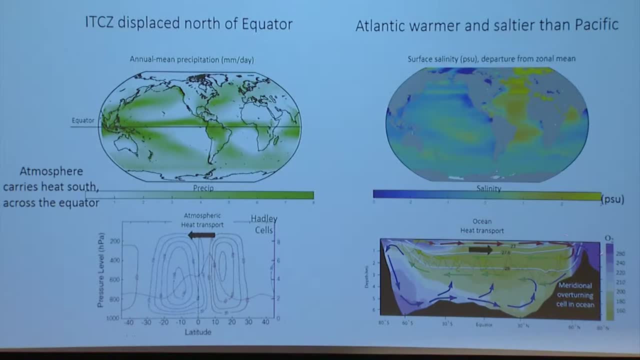 in which we get sinking. This is a section through the ocean. This is the equator north-south, This is the top few kilometers of the ocean. We get a great big overturning cell emanating from the North Atlantic which carries warm water across the equator. 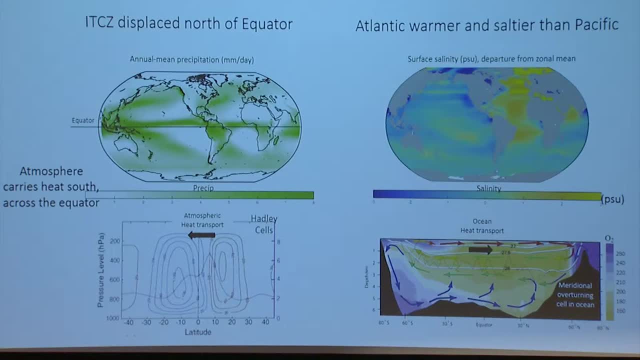 and we get cooling here and it returns at depth. This carries energy from the southern hemisphere into the northern hemisphere and plays a role in this, in this asymmetry. So these gross, large-scale inter-hemispheric and zonal asymmetries of climate. 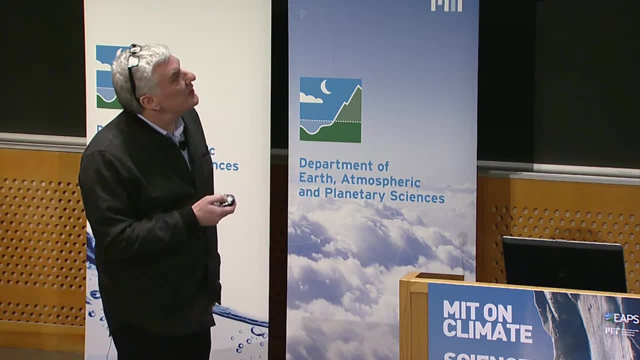 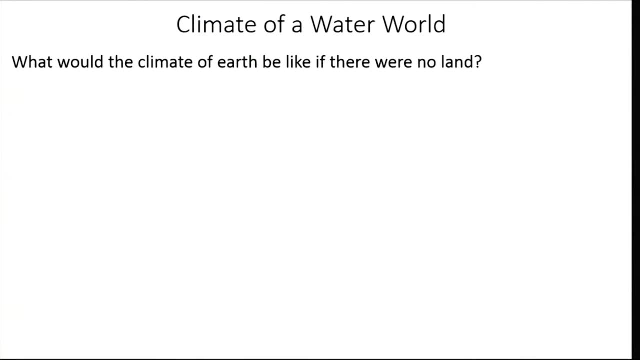 the ocean is playing a critical role in these patterns. So what I want to do is: You may think this is a bit of a bizarre thing to do, but I am an oceanographer, so what I'm going to do is actually try to build. 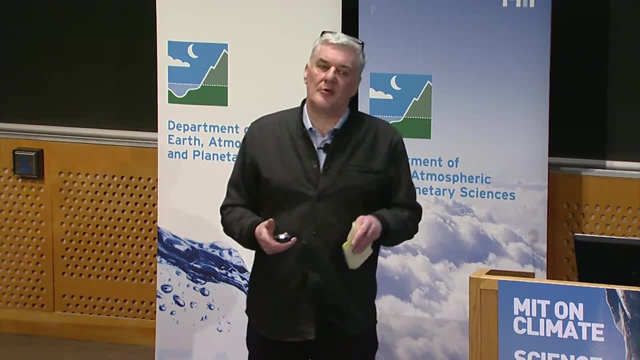 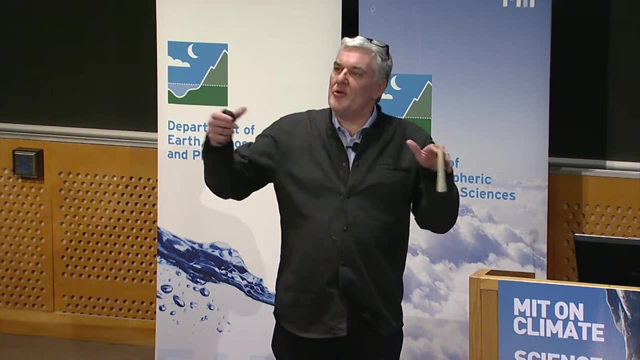 a cartoon of the climate system. I'm going to try and build a system which starts very simply and I put in a little bit more complexity until I get something that looks quite a bit like the real climate. And I'm going to start off. 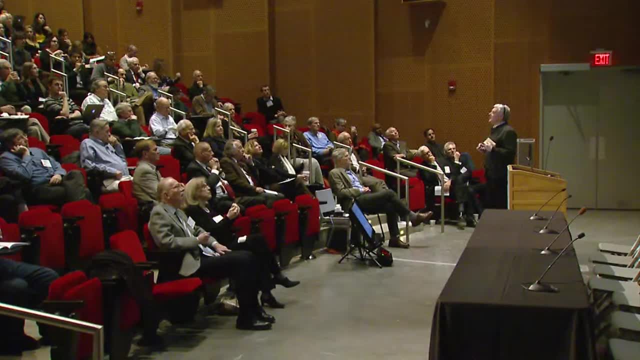 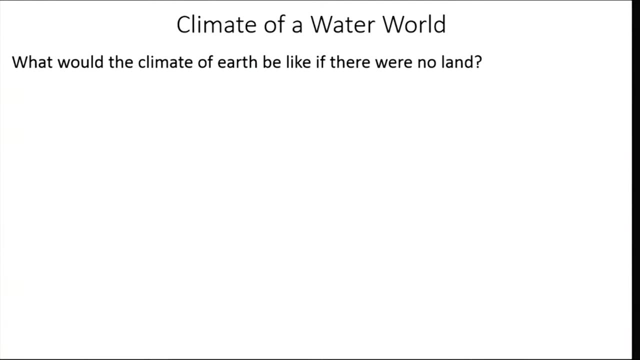 by just thinking about a world in which there were no land at all. So I'm going to look at the climates of water worlds and what would the climate of the Earth be like if there were no land around? So here is this world. 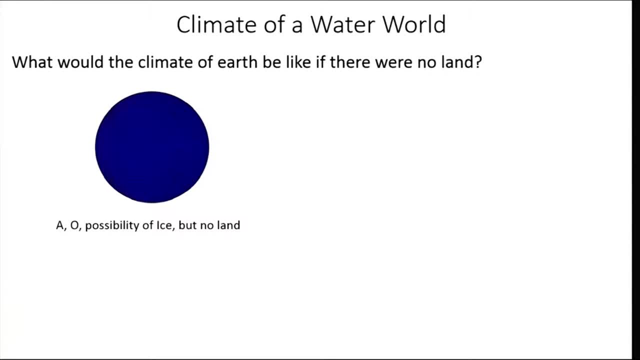 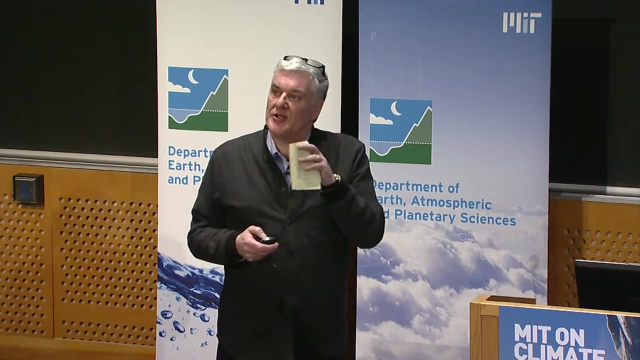 There's no land. There's an atmosphere, an ocean, the possibility of ice, but no land, And that's a simple system that you can think about. But one of the things that we see, One of the things about the ocean, is that it's in ocean basins. 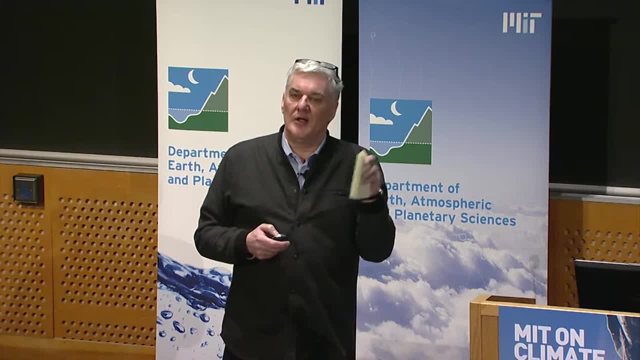 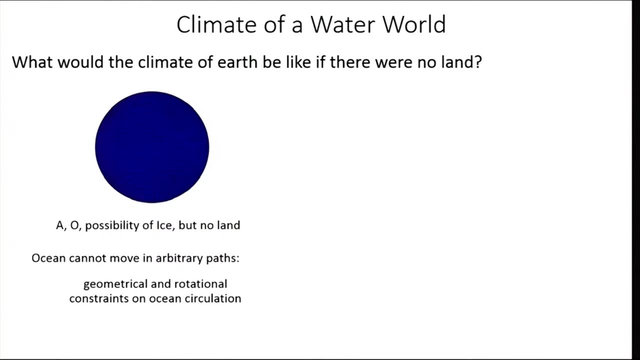 so it's constrained geometrically by coasts, And so the ocean can't move in arbitrary paths. There are geometrical and rotational constraints on ocean circulation, Rotation, meaning Earth's rotation, So we can put this kind of information into this system by introducing barriers. 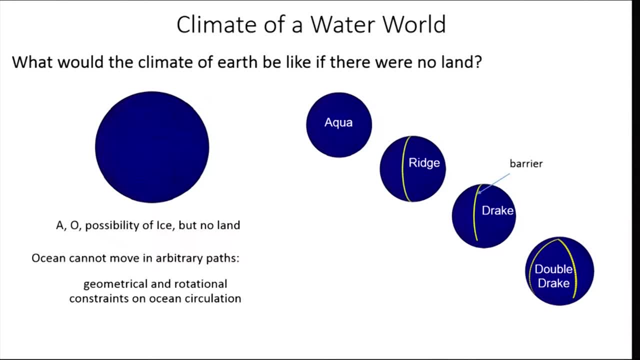 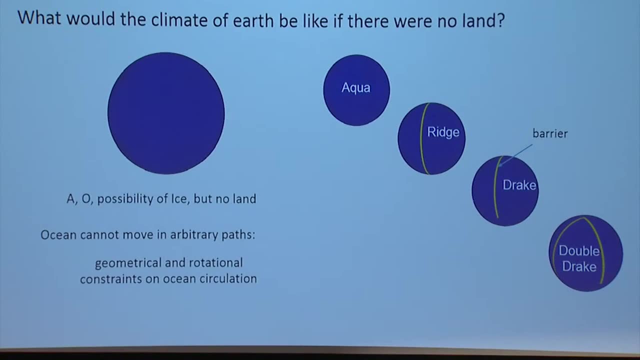 So I'm going to consider an aqua planet which is a pure aqua planet. It's an ocean which is a few kilometers deep, with a flat bottom and no land, And then I can introduce a ridge which is a barrier going from the North Pole to the South Pole. 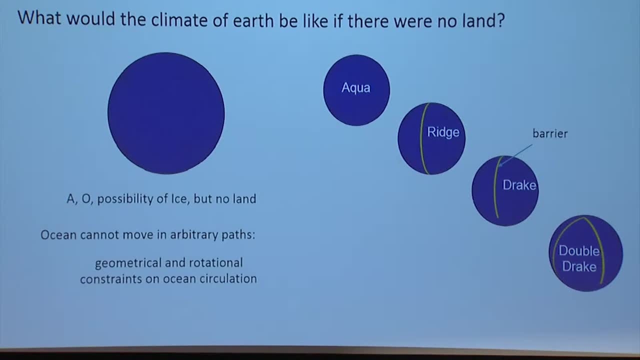 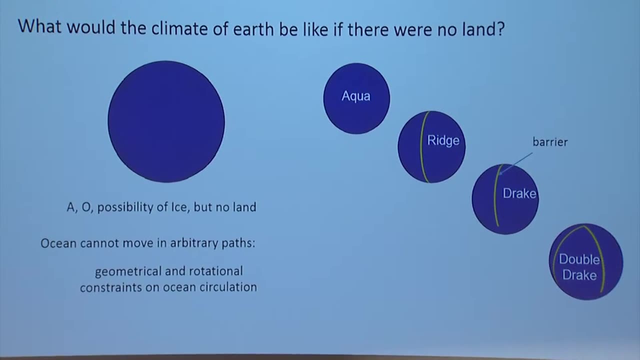 And look to see how the climate changes if I stick a ridge into the system And then I can open up. I can open up a Drake Passage by putting a gap in the barrier, Or I can have. This is my most realistic simulation. 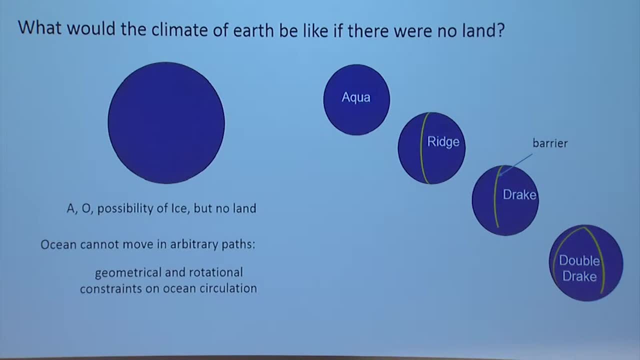 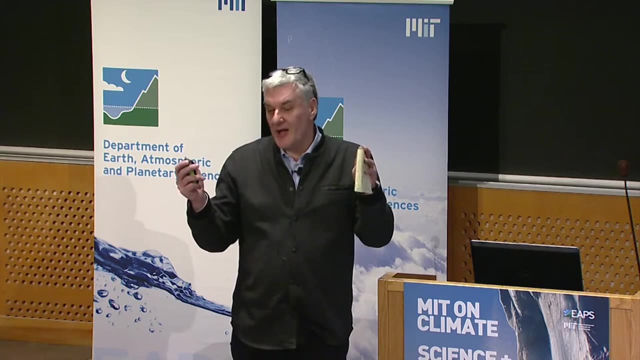 I have a double Drake, which is- But I actually get something that looks quite a lot like the real world. I have a double Drake which is a small basin, ie the Atlantic, and a large basin, which is the Pacific. 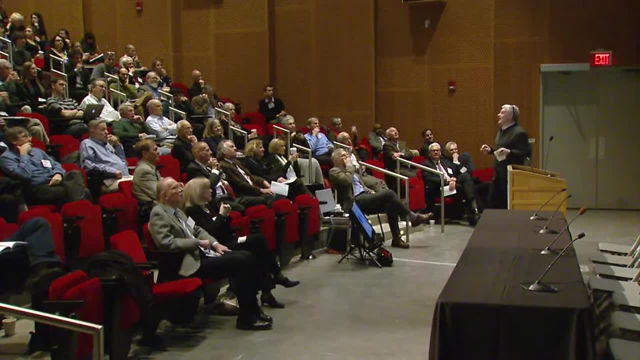 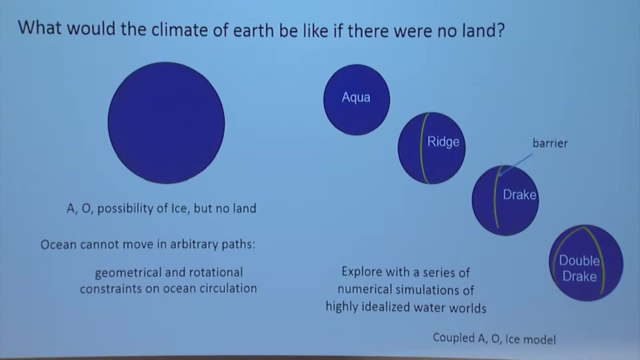 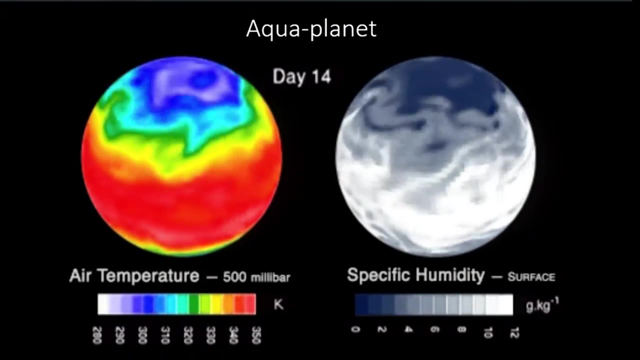 So I'm going to do this numerically, I'm going to explore this with a series of numerical simulations of these highly idealized water worlds and see if I can build up something that looks a bit like the real world. So here's my aqua planet simulation. 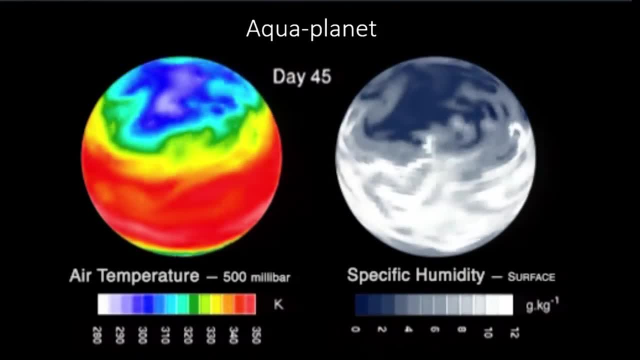 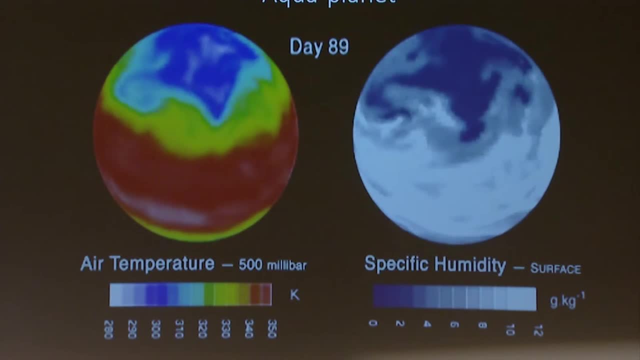 On the left we have the temperature at 500 millibars in the atmosphere, which is about five miles up. The red areas are warm, The blue area is cold. These are our weather systems and synoptic systems in the numerical simulation. 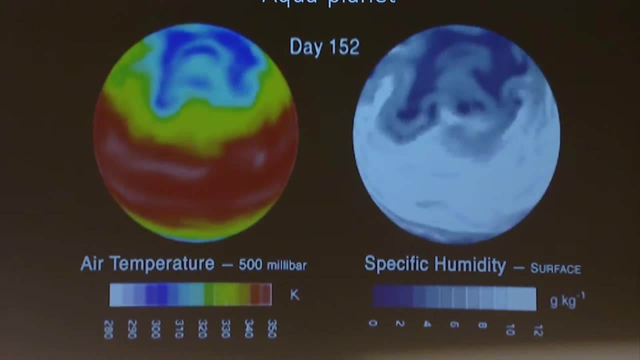 Warm air tends to be moister than cold air, so the whites are the humidity and cloudiness in the atmosphere. So we have more moisture in the tropics, less over the poles, And we integrate this system out for 5,000 years. 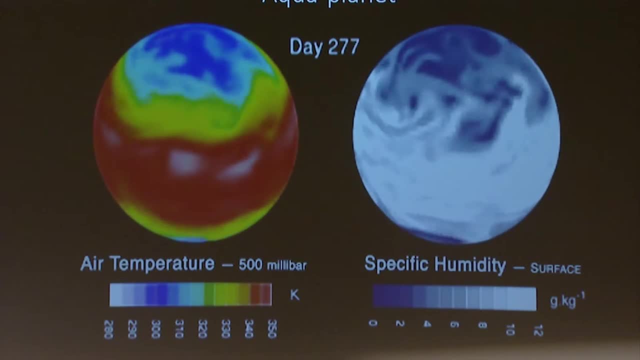 It's blowing over the ocean and the ocean's moving around and we're getting a coupled simulation. So this is day 300.. We have to integrate a long time because the ocean's a bit like an elephant: It kind of remembers things for a long time. 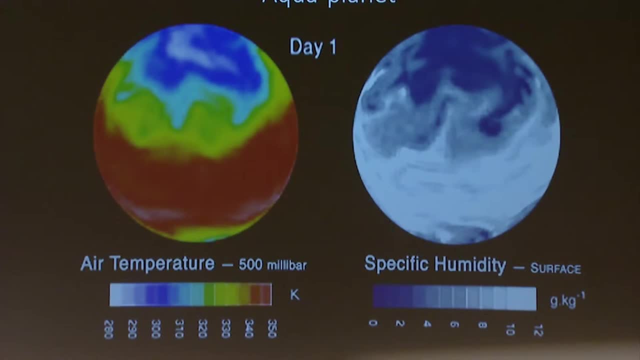 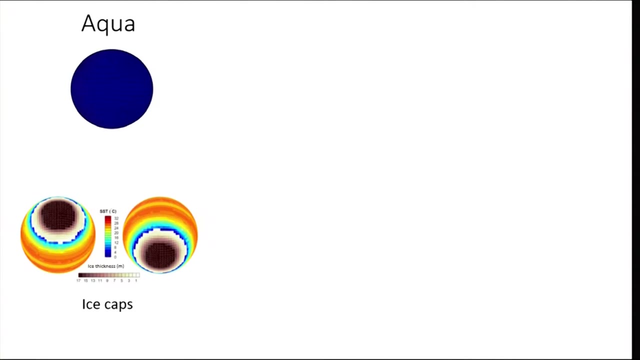 It takes thousands of years to mix itself up. So in the pure atmosphere, so in the pure aqua planet. if we do this simulation, we end up with two ice caps, one over the northern hemisphere and one over the southern hemisphere. This is sea surface temperature. 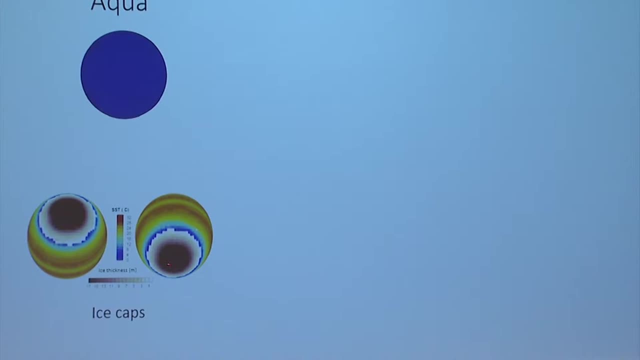 in the climatology of this simulation, I've got an ice cap here and an ice cap there on my pure aqua planet, And the reason for this is that the ocean, because the Earth's spinning around, there are angular momentum constraints on it. 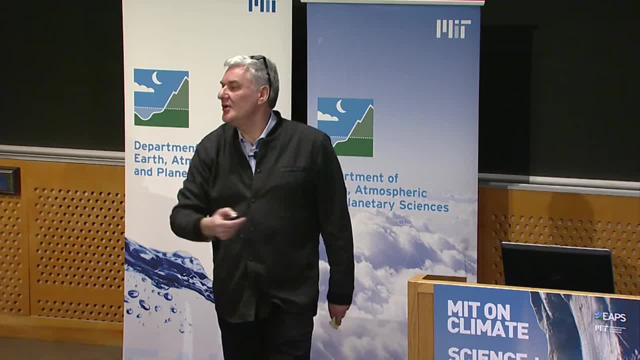 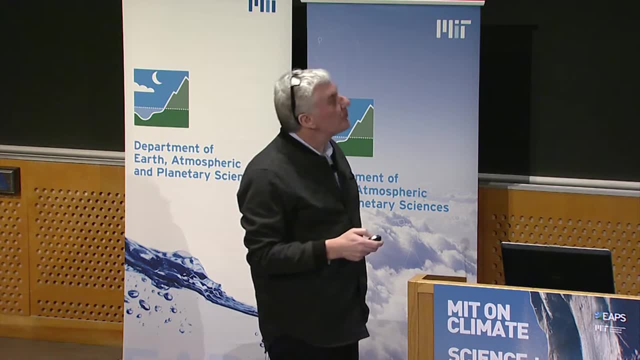 so the ocean kind of moves along. It moves along in zonal currents and it can't get energy to the poles very easily, and so we get these big ice caps. But now, if I put a ridge in the system that connects one pole to the other, 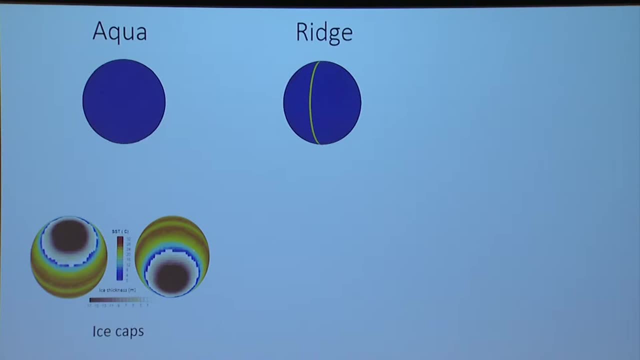 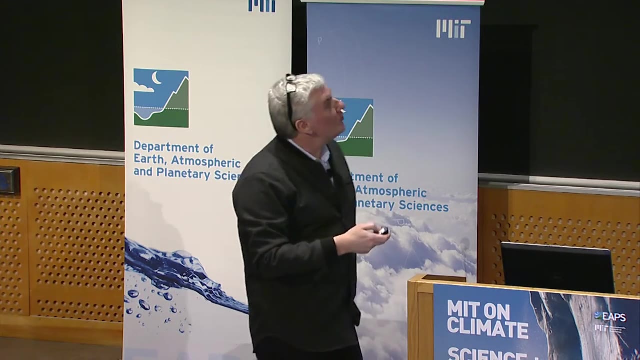 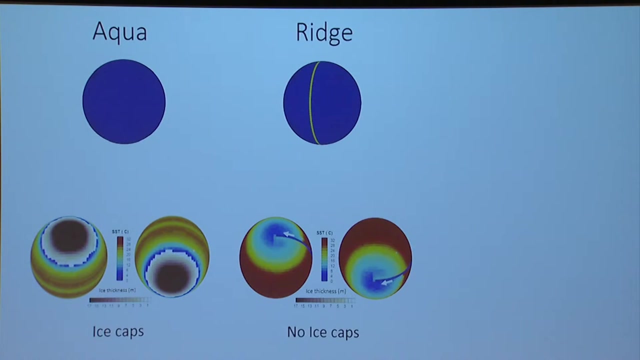 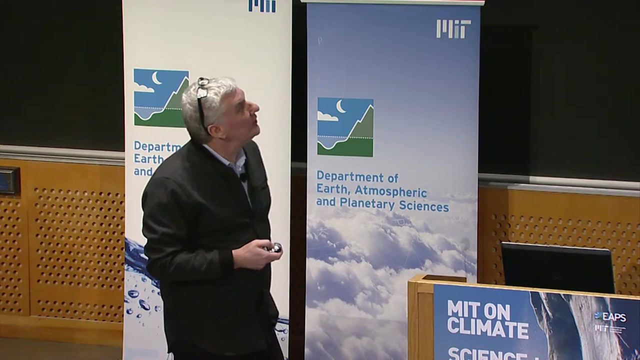 what do you think happens? The ridge is an assist, and it enables the ocean to move energy to the poles, And so what happens is that we get no ice caps in this system, So the ice goes away. in this system in which we have a barrier going from one pole to the other, 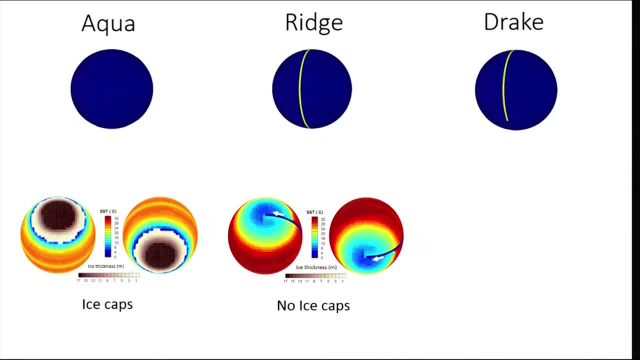 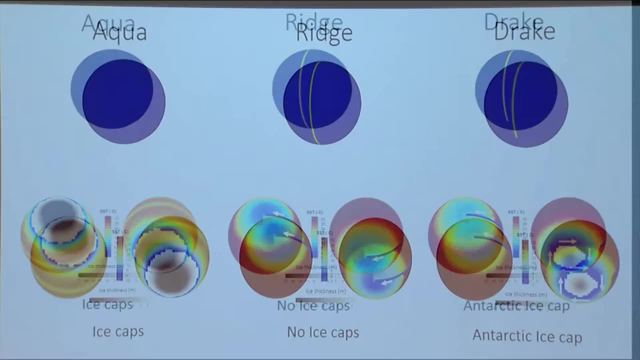 Well, what happens in the Drake simulation? Can you imagine what might happen? You get an Antarctic ice cap and no Arctic ice cap. So in this way we're able to build up this very important interhemispheric AC asymmetry in climate. 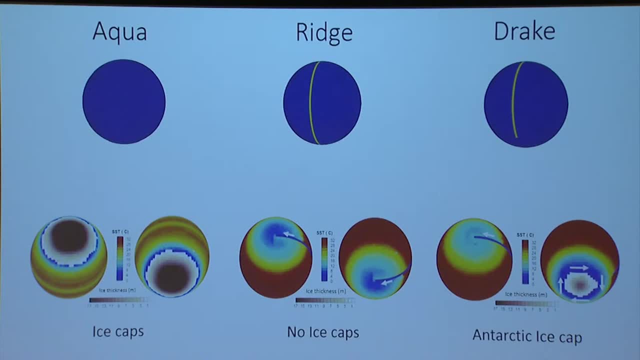 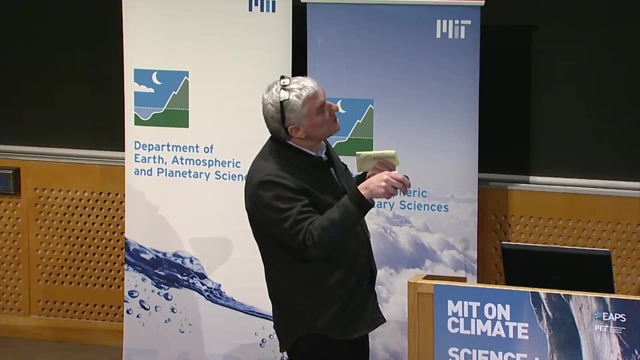 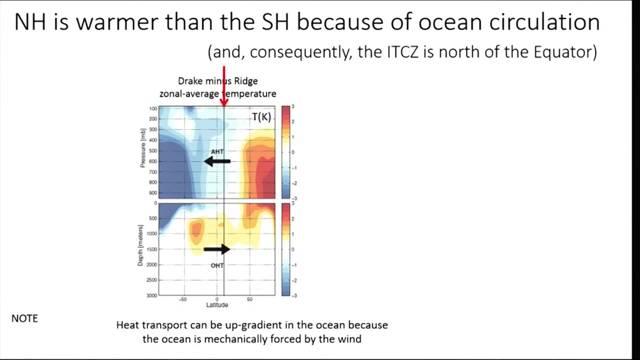 ie the southern hemisphere is colder than the northern hemisphere and there's a great big ice cap over Antarctica and no ice cap in this particular simulation. with the Drake You can go further and look again at the Drake minus ridge and look at the interhemispheric asymmetry. 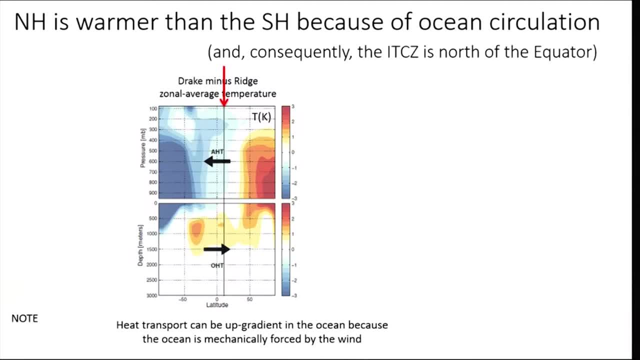 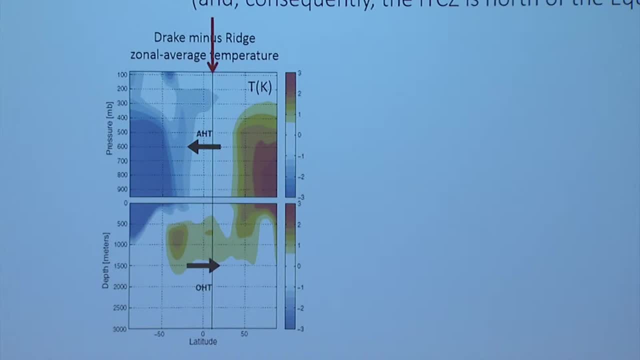 in temperature. This is the asymmetric temperature distribution. It's warm in the northern hemisphere and cold in the southern hemisphere, And what the ocean's doing in this Drake minus ridge is it's carrying energy. The ocean is carrying energy from the southern hemisphere into the northern hemisphere. 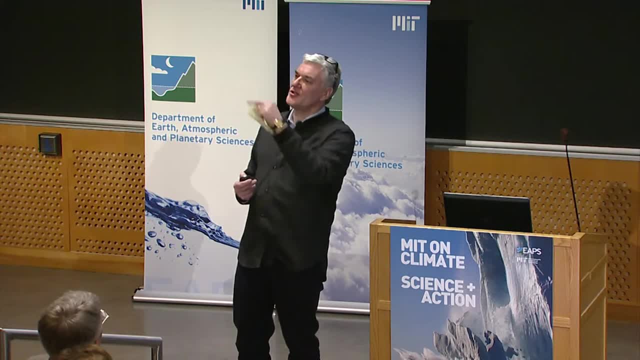 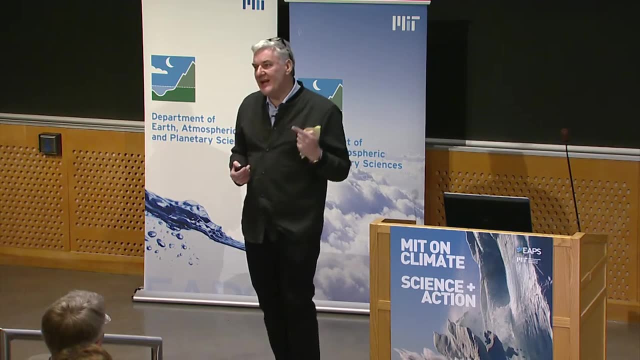 And it's actually carrying it up gradient. It's carrying it from cold places to warm places. The reason it can do this is that it's mechanically forced. It's not working like a heat engine. It's mechanically forced and so it can actually carry energy up the heat. 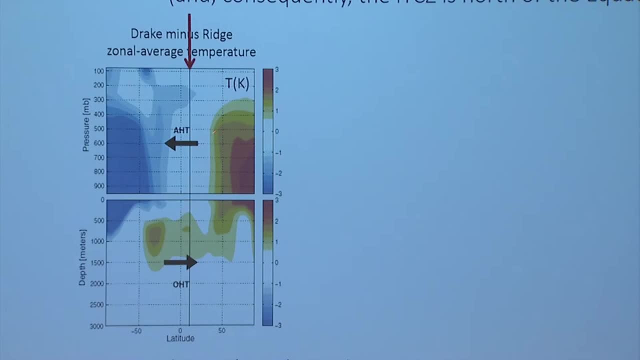 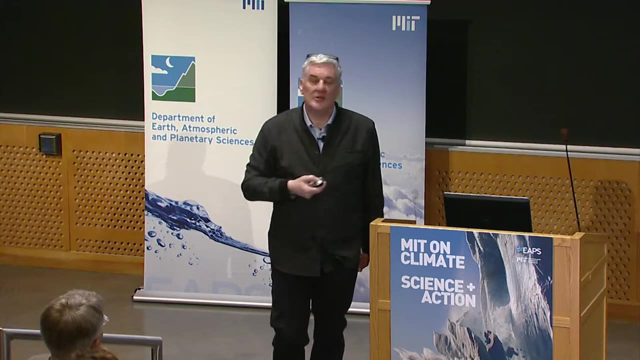 up the temperature gradient And the atmosphere is moving energy from the northern hemisphere into the southern hemisphere, and it does that by shifting the ITCZ north of the equator. I don't have time to show you this, but the intertropical convergence zone. 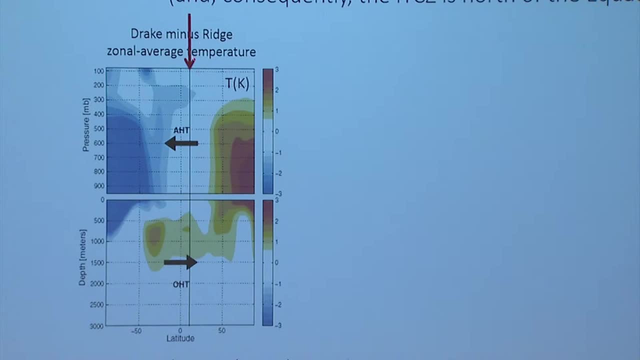 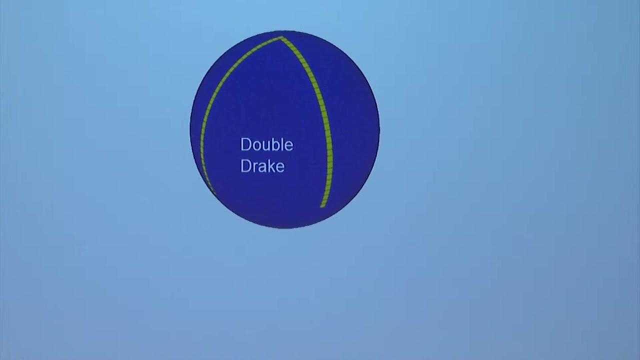 this band of cloud and excess precipitation is actually north of the equator. in this, in this model, And if I compare that with the, if I compare that with the observations, there are some broad similarities between the two. So now the high end of this hierarchy of models. 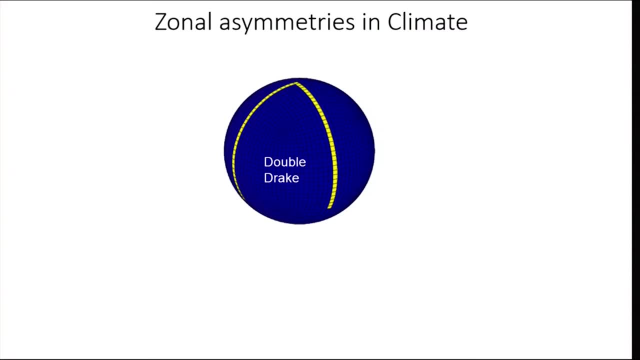 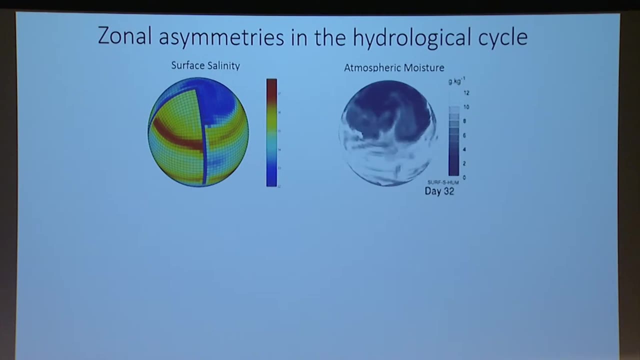 is this double Drake? So now I do the same kind of calculation, but I have a small basin and a large basin, And, and, and so what? what happens now is very interesting. So what happens is: so: this is the moisture field in the 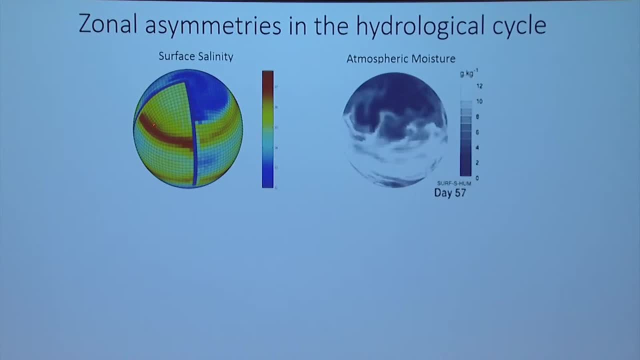 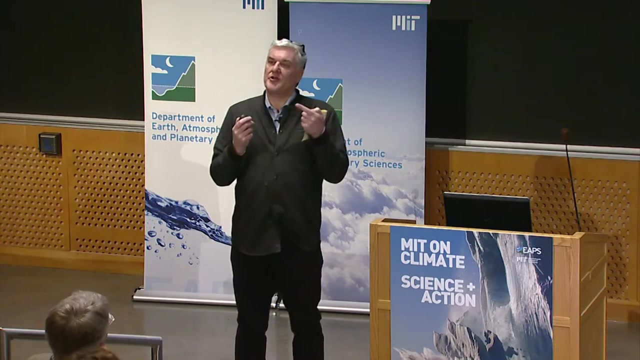 in this simulation And what happens is that the, the ocean tickles the atmosphere, so you get more weather systems being formed in this, over the small basin, because there are there are sea surface temperature anomalies associated with the boundary currents, So the storm track in the atmosphere gets organized. There's evaporation of water from the ocean in the small basin And it carries it zonally across and dumps it as as water over the large basin. So the large basin gets fresh and the the small basin gets salty And 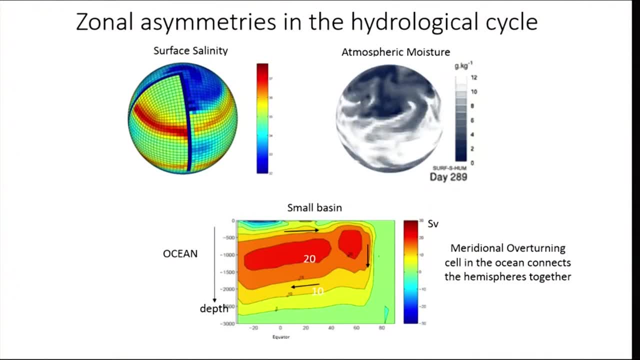 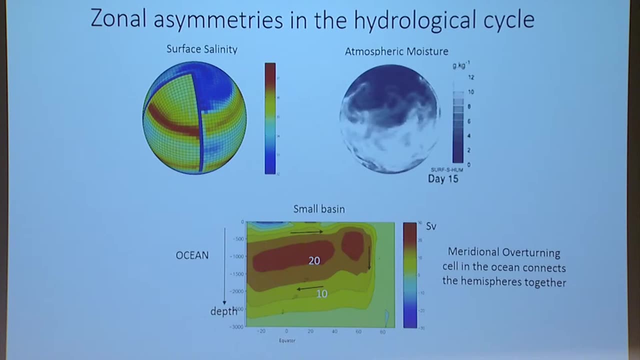 and and what. what we then see is that that the salty water is denser than than fresh water, And so you get convection in the ocean and an overturning cell, this conveyor belt, which ends up being confined to the small basin. 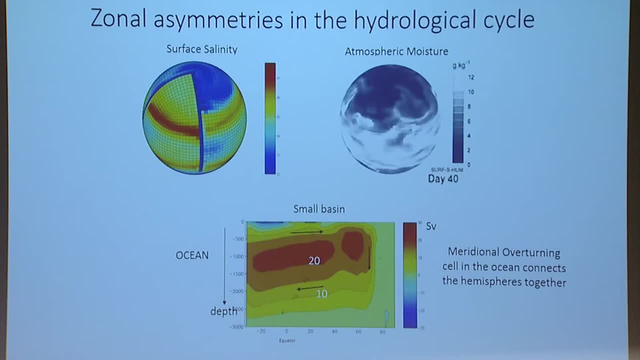 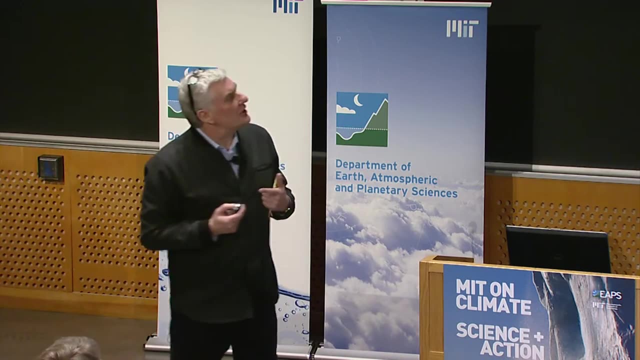 And so you get this. you get something that looks really quite a lot like the. I mean, if you, if you kind of take a bird's-eye view of this, it looks quite a bit like the, the present climate, And you can go further. 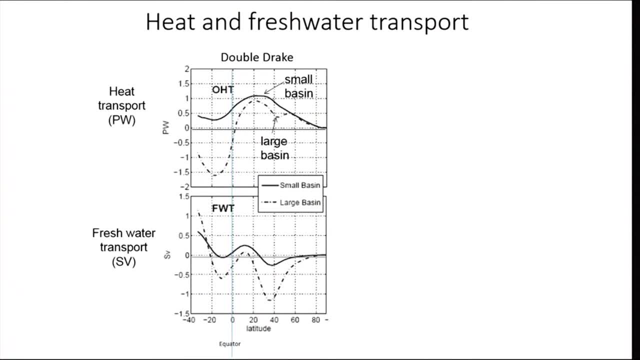 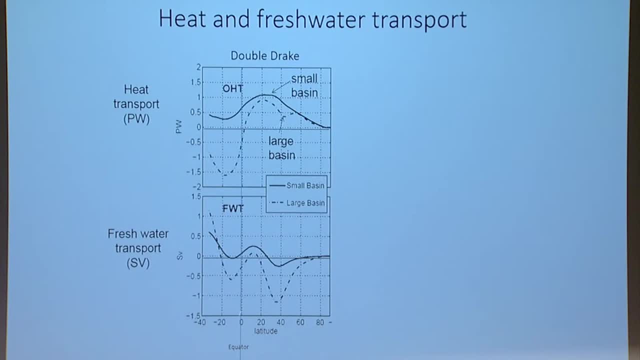 and look at the heat and fresh water transport in this, in this system. So this is the meridional energy transport in as a function of, of, of latitude. This is the equator moving northwards. This is in the small basin. 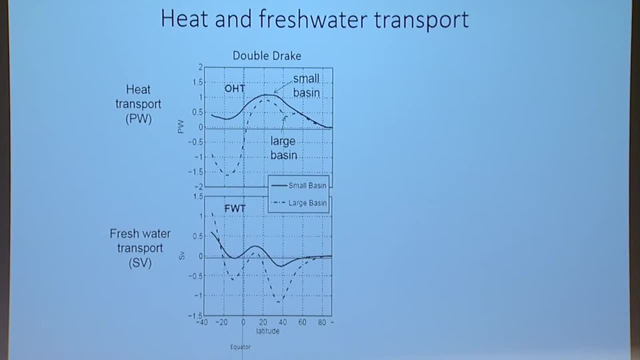 So this is the transport of energy across the equator, from the south to north, which is in petawatts- This is an order 10 to the 15 watts per meter watts going across the equator. This is the large basin. 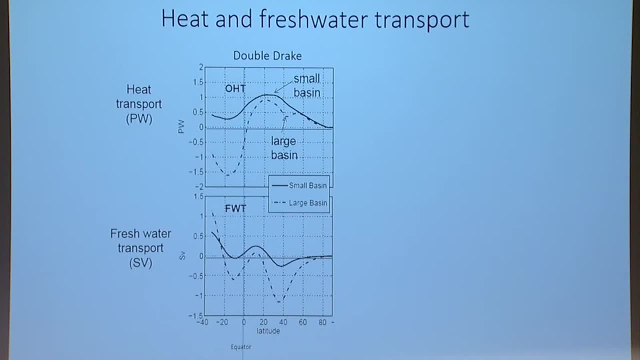 This is the fresh water transport. I don't have time to go into these details, but now, if I compare this to the observations, this is the actual observed transport from data, or inferred from observations. There's a striking similarity between the two, which tells us that really. 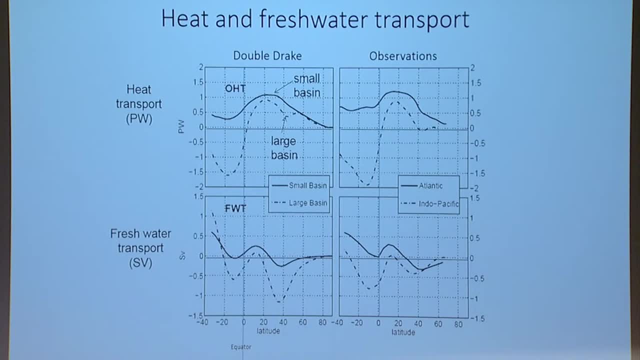 the land doesn't really matter in this regard- Actually, it does matter to some degree, But we've been able to in a cartoon-like fashion. we can construct a world that looks a little bit like our present by just having a few sticks. 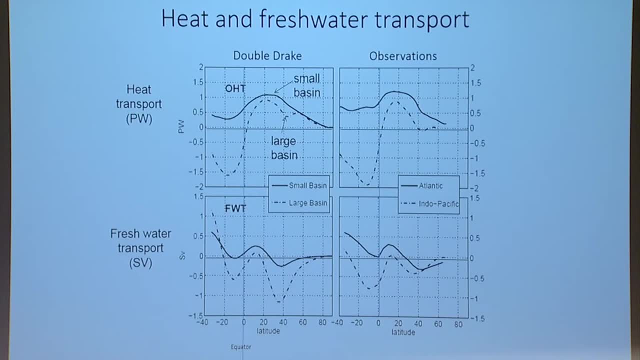 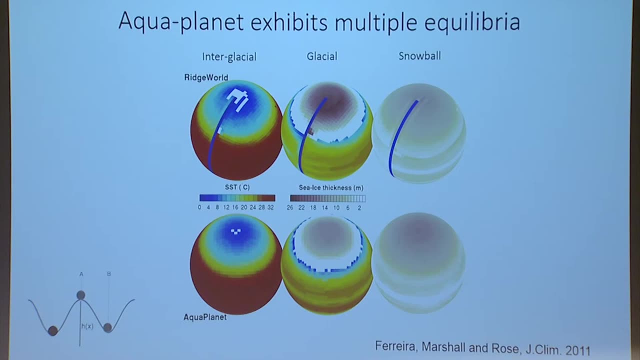 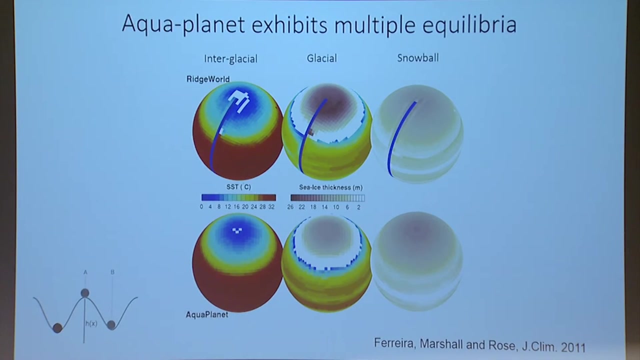 in the in the ocean. Now this aqua planet exhibits multiple equilibria. This is a really fascinating thing, And it gets back to some of the work that David McGee was reporting on, that the Earth has been in many different states. 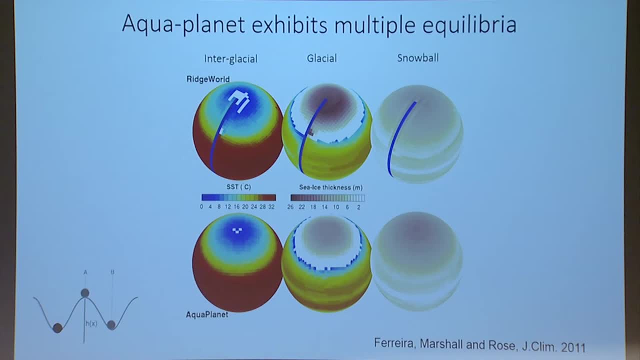 It's been in hothouses, It's been in glacial, We've been in glacial climates, We've been maybe even in a snowball 800 million years ago, And the remarkable thing is that both the ridge world and the aqua planet 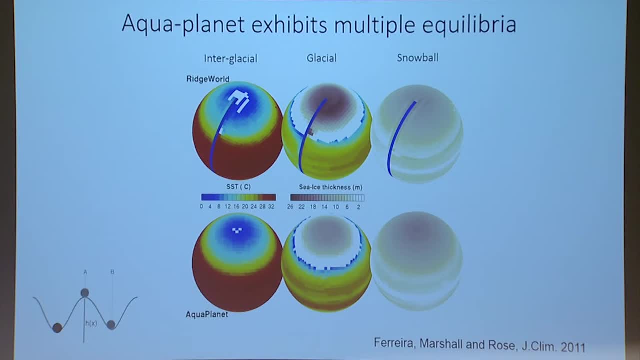 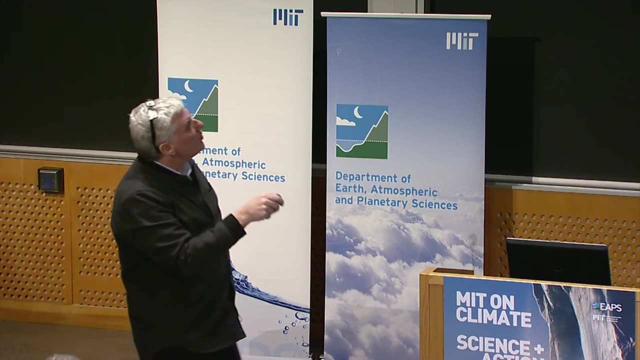 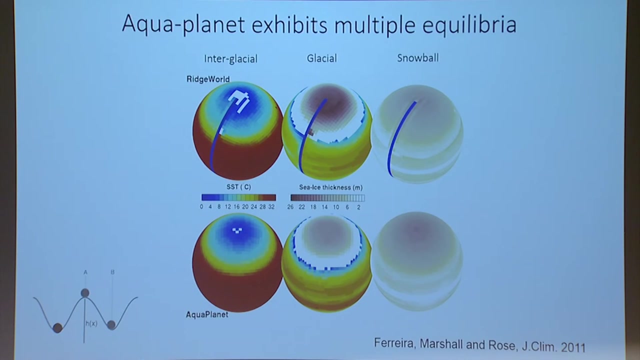 exhibit multiple equilibria in the sense that, if we use the same forcing the model, We can maintain three different climate states: one which is warm, one which is a glacial state and a snowball where the whole planet freezes over. 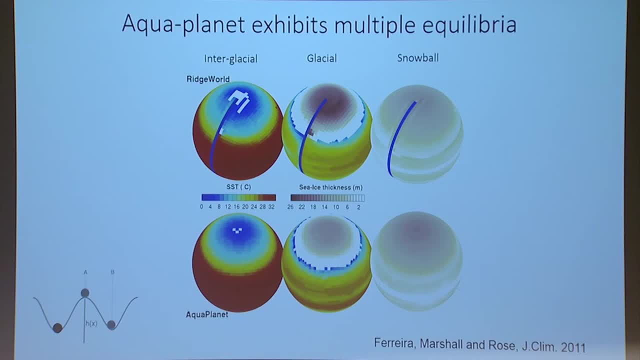 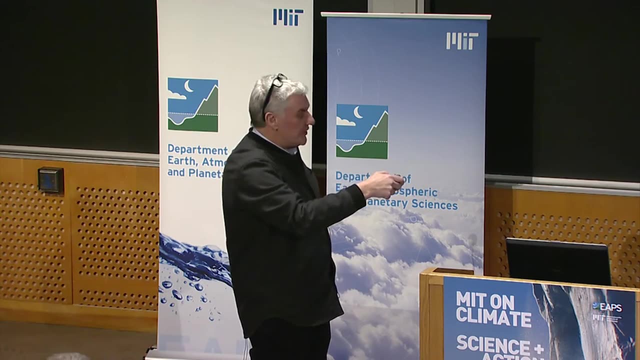 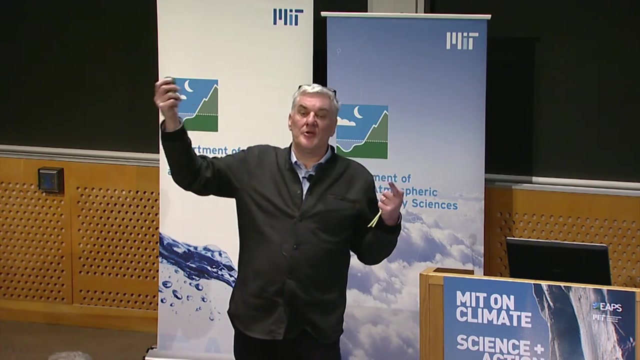 And these are. These are multiple equilibria in the sense that you've got a ball rolling around a corrugated surface, and they're equilibrium states. So one of the questions that one might ask is: could Earth flip into another state? 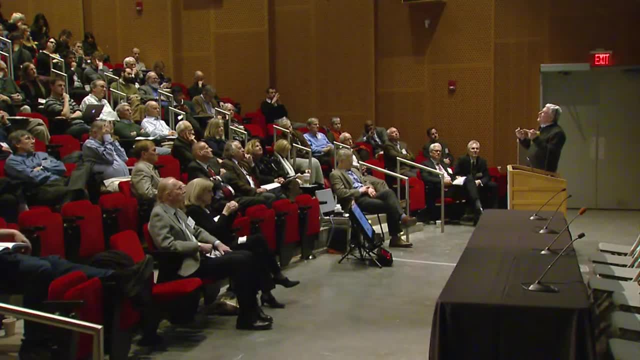 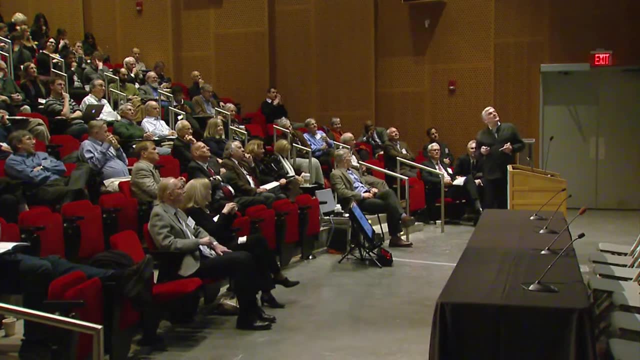 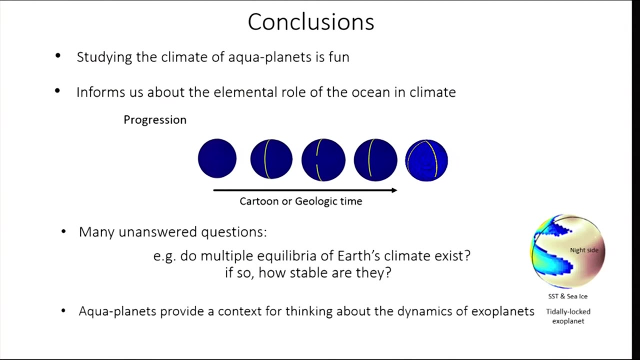 Are multiple equilibria a way of thinking about past climates? Have I got zero minutes? Yeah, So good Conclusions. So studying the climate of these aqua planets is fun. I've become obsessed by it, for, And I'm now reluctant to put land into the system. 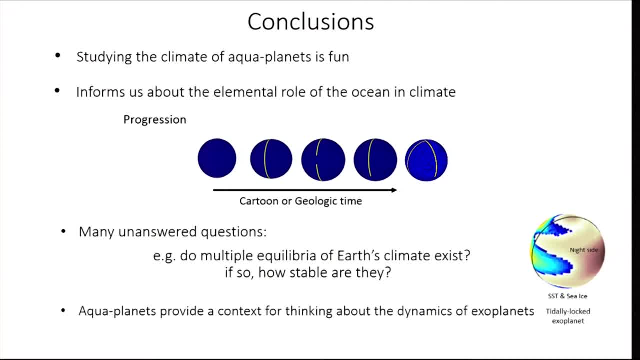 It informs us about the elemental role of the ocean in climate. So we can think of this progression as a cartoon of the climate. If I wanted to draw a cartoon, what would the essential things be about the present climate? So it would be inter-hemispheric asymmetries. 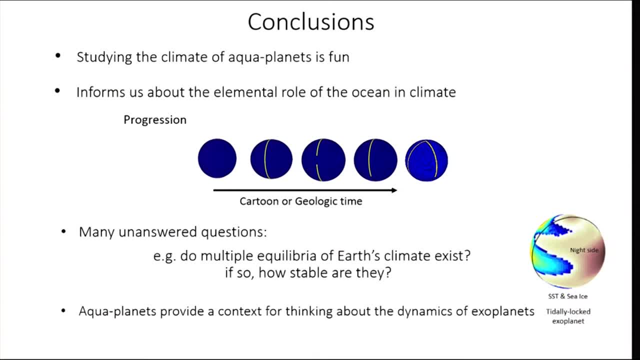 geometrical ones and zonal asymmetries. We can also think about it as an evolution over geological time. You know, as the plates move around the world, you know we move into We, The tectonics drives the land into these. 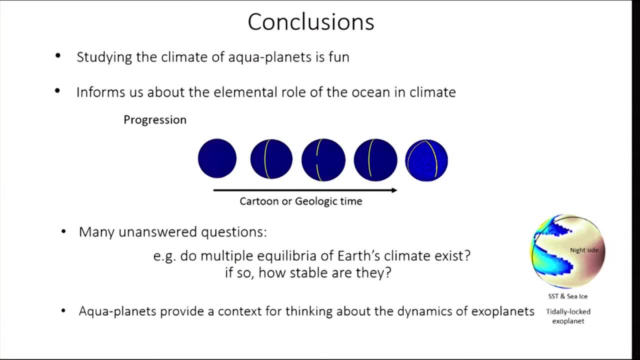 into this evolution. There are many, many unanswered questions. Do multiple equilibria of Earth's climate exist? They do in this model. If so, how stable are they? And we can also use these kind of calculations as a framework for thinking about the dynamics. 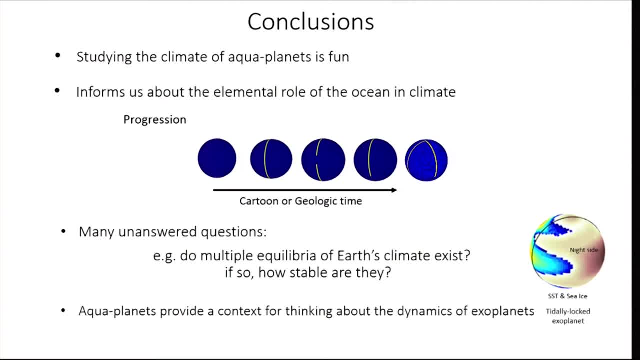 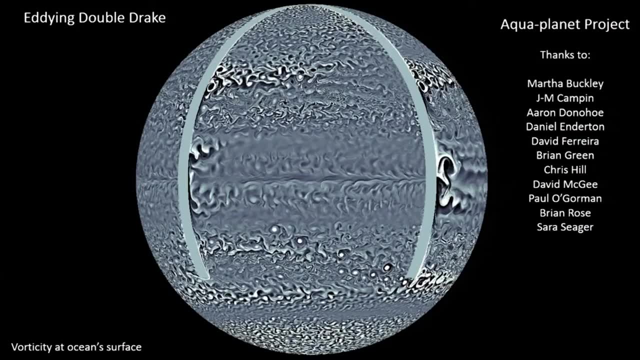 say, of exoplanets. We've been working with Sarah on these matters, So, And I'm going to finish off by thanking lots of people- Thank you, And thanking lots of people who, over the years, have been working on these kind of. 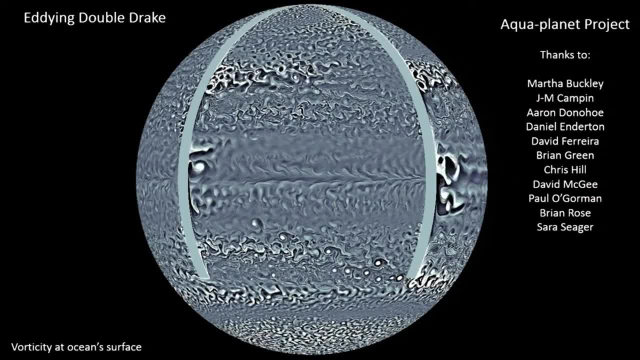 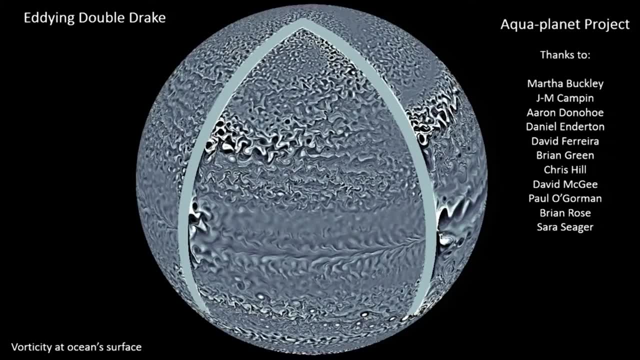 on these kind of problems. This is a very high resolution simulation of an aqua planet, So this is what the ocean would look like if North America were shrunk to a. I've got to stop. Thank you very much. Thank you. 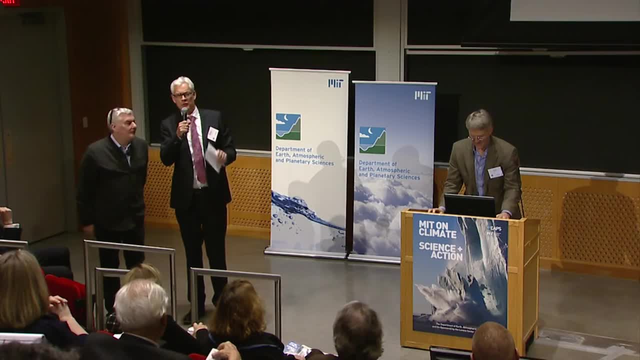 Feels like an AGU meeting in the confine here. This is exactly why the geologists and the oceanographers love each other in our department Looking at the rocks, But your sticks, of course, are the continents and they move all about. 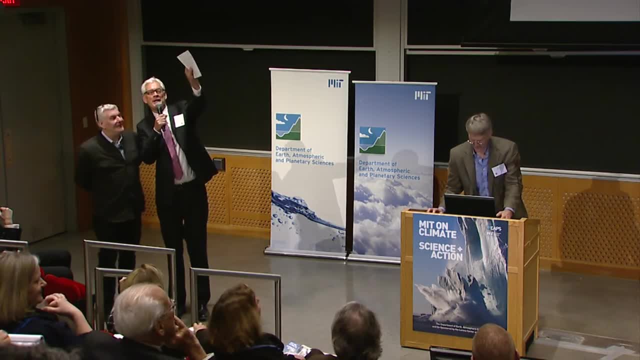 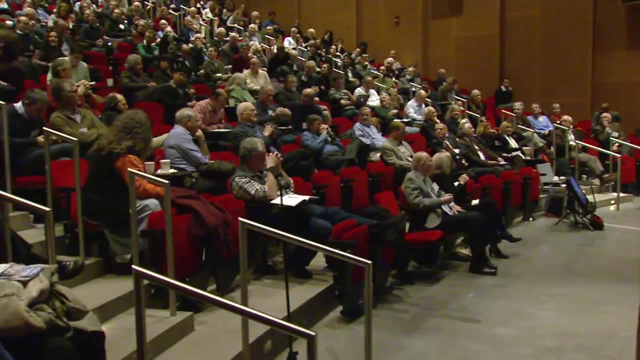 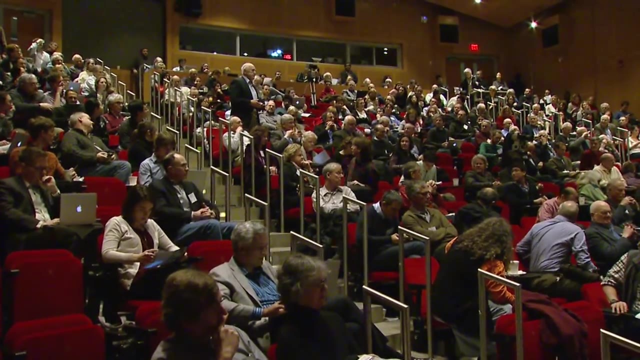 So it's all about land, and Anyway, One question and then we have to move on. Victor Starr's main contribution to the dynamics of the climate was that most of the interesting energy motions are upgraded. He summarized that in a book he wrote on the physics of negative viscosity phenomena. 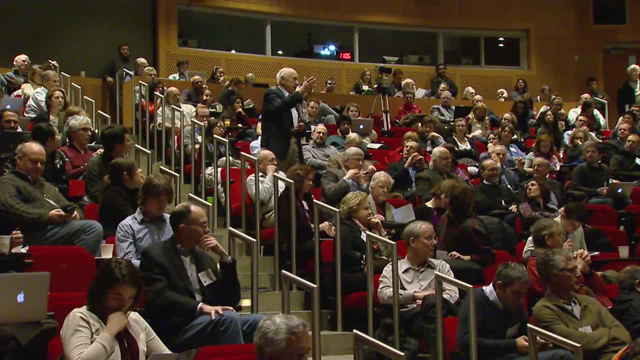 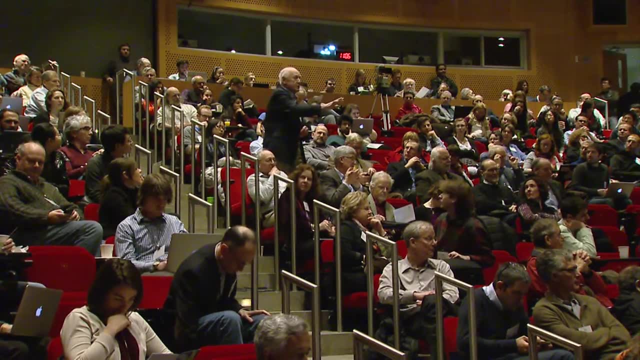 Yes, You said that you had to put in a ridge in order to get upgraded transports, but you don't. What Victor Starr said is: you can get those anyway Now. the ridge may help it, but it isn't necessary. Okay, so the question was: 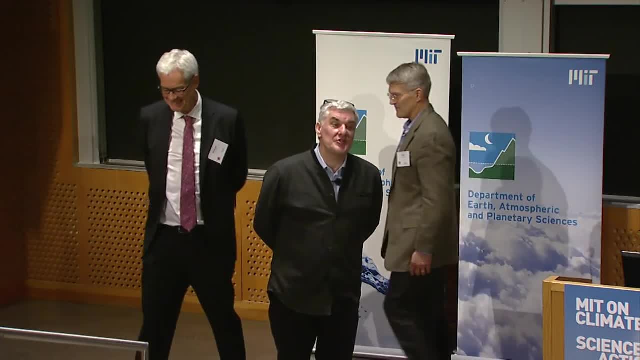 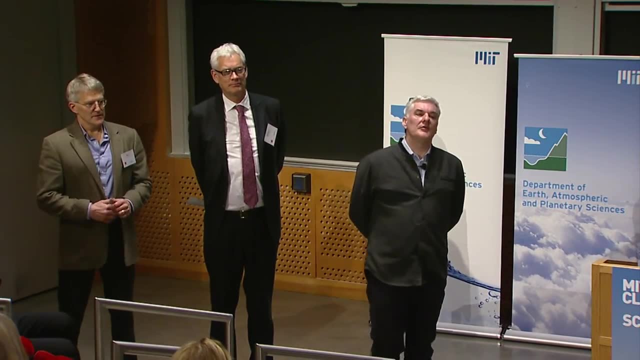 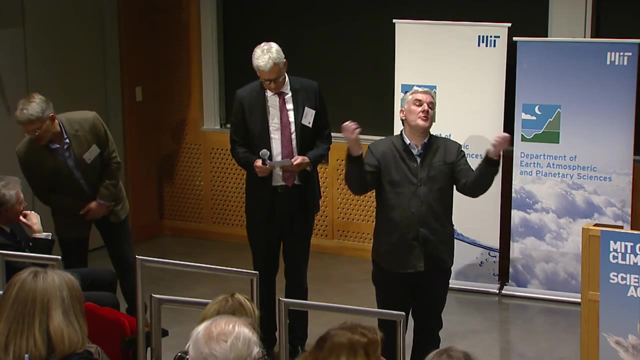 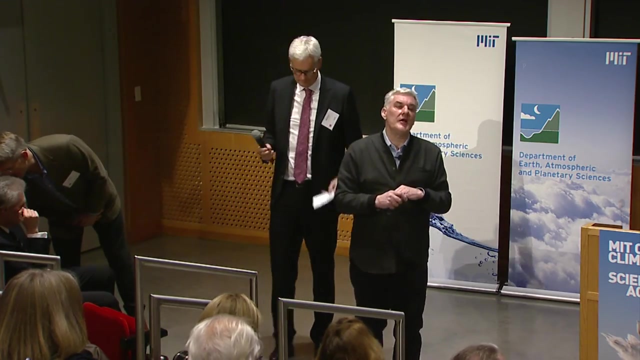 can. any Momentum is transferred up gradient. Victor Starr was talking about momentum. I'm talking about heat. The atmosphere takes heat down gradient. It's thermally driven and it can transfer momentum up gradient And Victor Starr realized that. Not always, but Victor Starr understood that. 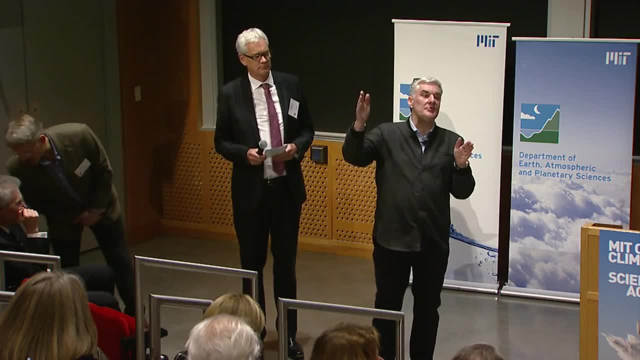 The ocean can actually transport heat up gradient because it's mechanically forced. That's a different thing.